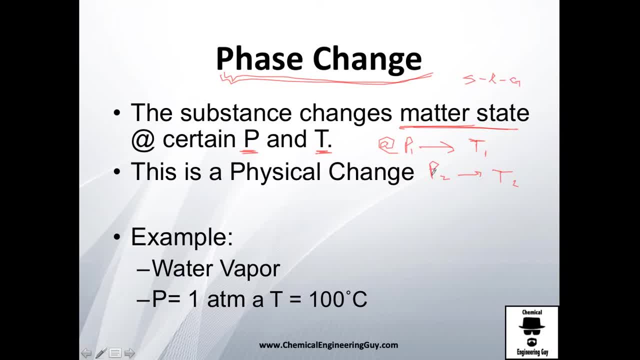 going to study that in the next slides. but just take into consideration that for every temperature you say you need to have a pressure. For example, you probably know that water boils at 100 Celsius, but I always tell my students and all the people that say that that they must. 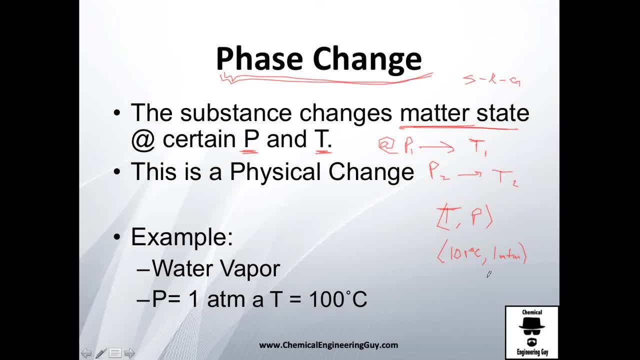 specify at one atmosphere, because you can even boil water at 90 Celsius at lower pressures. So it's kind of obvious that when you say 100 Celsius is at one atmosphere, but the most thermodynamic correct phrase will be at certain pressure. Very important: this is a physical change, not a chemical one. So the pure 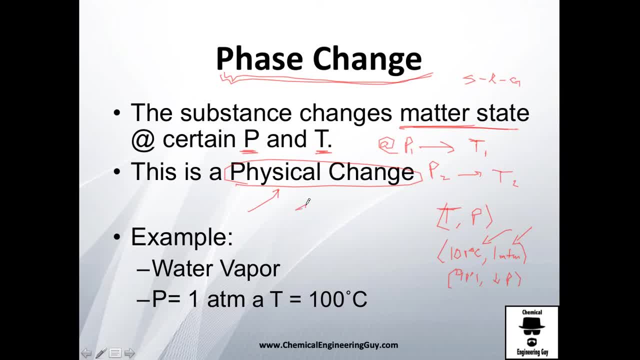 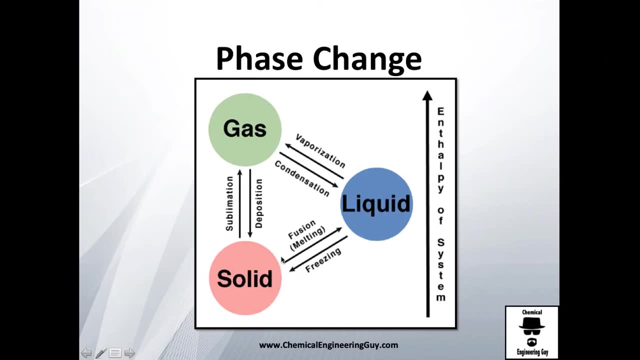 substance is still being the same. pure substance, For example water, is still H2O, even though it's gas, vapor, or liquid or solid. Whatever the case it is, the composition is the same. Okay, so remember that enthalpy, remember that H2O. 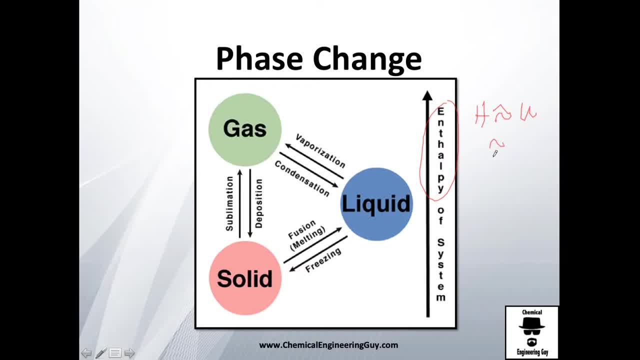 which is similar to internal energy and which is directly proportional to the temperature. As you can see, the higher you go from solid liquid and gas, you increase the enthalpy. Enthalpy means essentially energy, So we could say that this is not enthalpy, but also. 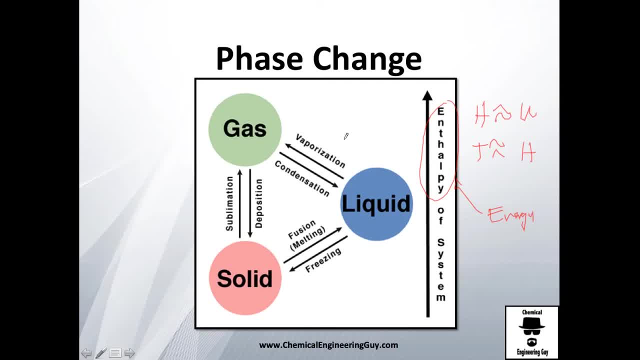 energy. So see that arrow: as the system solid, changes to liquid and liquid, changes to gas, The energy also increases and of course, if you condense something to liquid and then freeze it, you're going to lower the energy on this system and you can see. 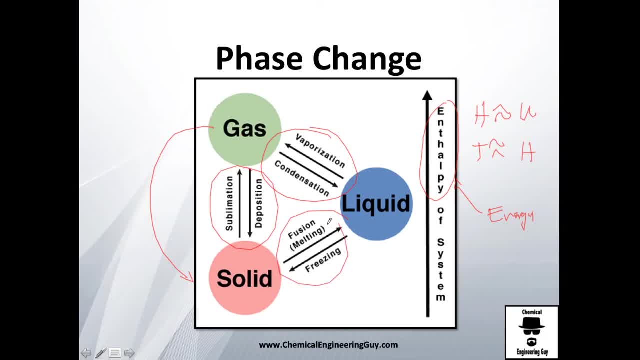 the changes or the what's the name of the process when you change from solid to gas. it's sublimation. it's kind of interesting. probably, you know, if you go to the bathroom- especially men- they have these pills that are for nice aroma and it's nice because they are solid and they go directly to gas to have a good. 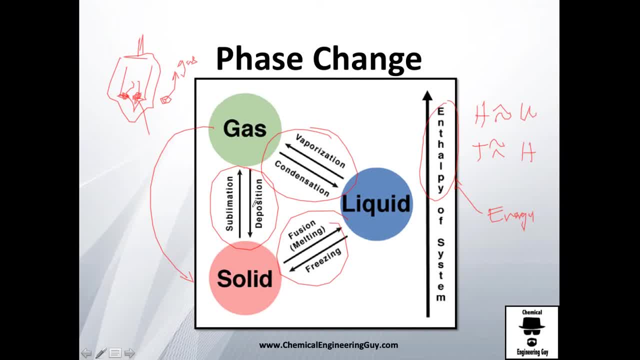 aroma, good smell, etc. the position: it's a little bit more complex. I'm not going to explain that, but will be. if you're in a gas phase, they go directly, directly to depose on the surface and they are solids. probably you're used to solid liquid, which is diffusion, or liquid to solid, which is freezing. gas to liquid is. 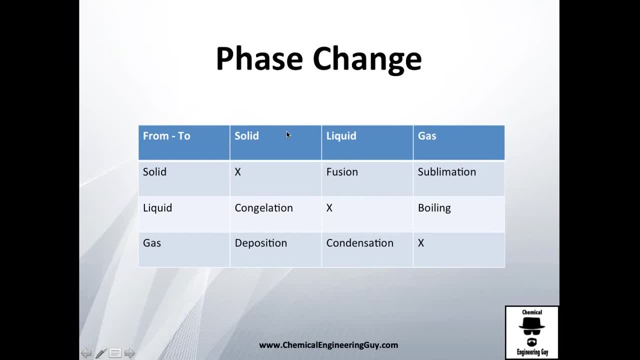 condensation, and liquid to gas is vaporization. so I bring you this table. it's a little bit more logic. I love this. solid to solid and liquid to liquid and gas to gas. of course they don't exist. this is no process at all, but solid to liquid, from solid to liquid, you will. 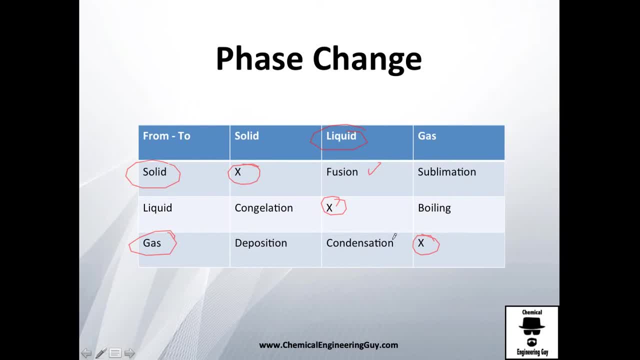 have fusion. from gas to liquid, you will have condensation and you can use a table whatever or whatever you want to choose. for example, liquid to gas, you will have boiling gas to solid. you have the position and I don't recommend you to learn it as a or learn by heart. just learn it by. 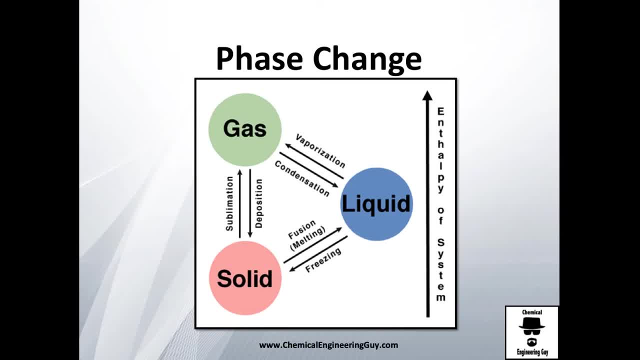 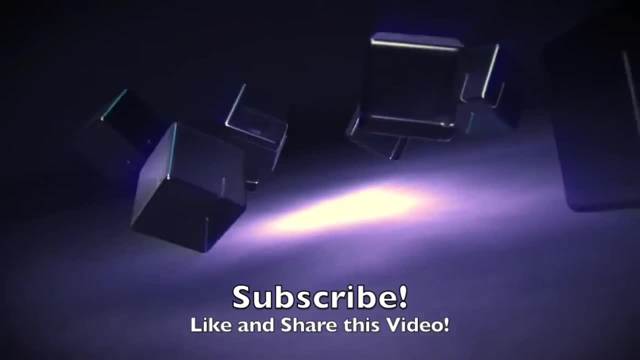 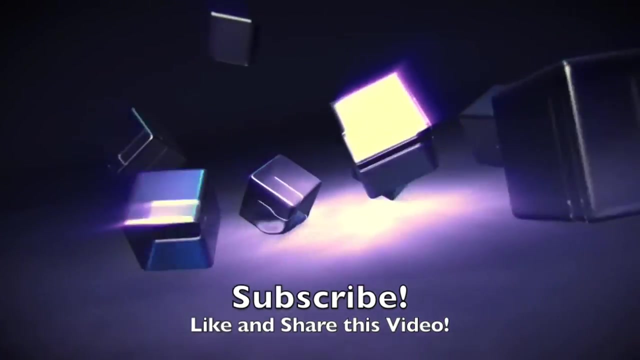 logic you know, probably gas to liquid and solid to liquid. maybe the only ones you need to learn are these two new guys right here, which we will not be using that much in the course, but it's thermodynamics. what's up, guys? it's me chemical engineering guy. so if you liked the 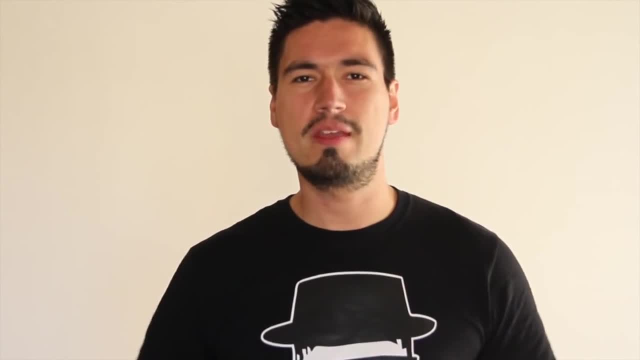 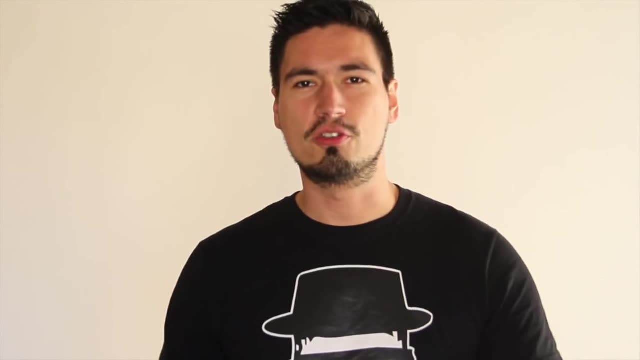 video. why not push the like button? it really helps me to know if you like in the videos or if I should be changing something or I should be adding something, taking out content. whatever also sharing is caring. so if you got any kind of friends, teachers, colleagues or whatever kind of person that might be. 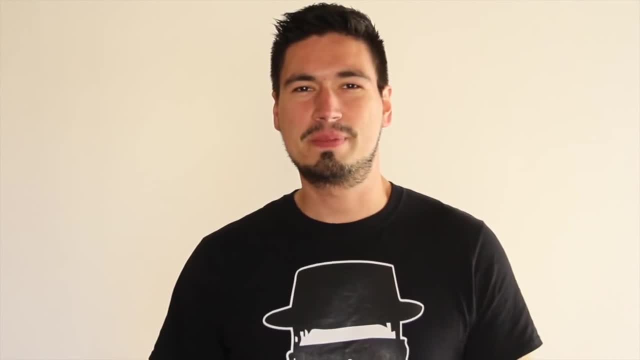 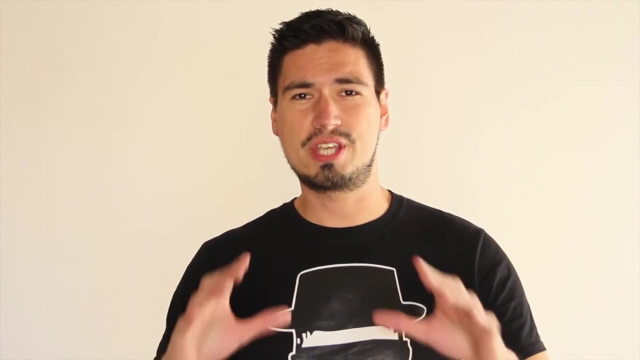 interested in this type of content, why not share it? sharing helps our community faster- in members and in content. if you want to keep track of my activity- videos, uploads, experiments, plays, whatever content I'm getting due- to be sure to click the subscribe button. subscribe to the channel is totally free, guys. my